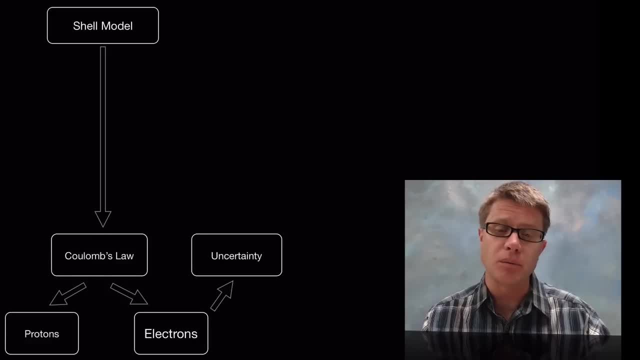 an electron. There's uncertainty there, And so they live in these clouds of probability. And so, since they don't follow specific orbits, we came up with this new term, which is an orbital, Which is where they're going to follow specific orbits, And they're going to follow. 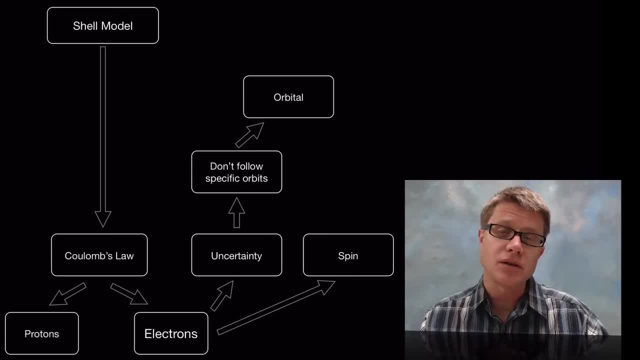 specific orbits And they're going to spend their time. Another important thing about electrons is that they have spin, So they're going to either have a clockwise magnetic spin or a counterclockwise magnetic spin And as a result of that, you can only have 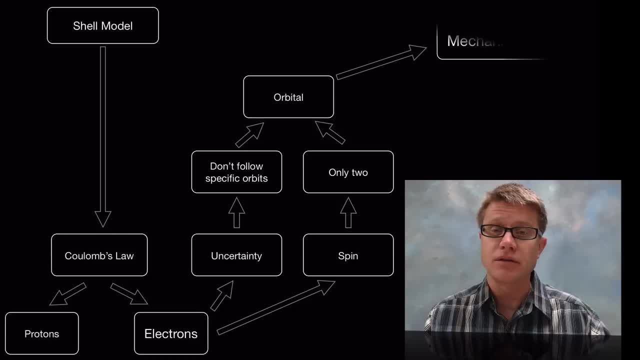 two in every orbital, And so we really had to throw out this idea of the shell, or at least modify it so it fit with the data. And so now we have this quantum mechanical model, And we can use complex equations and computers to develop software that predicts how atoms 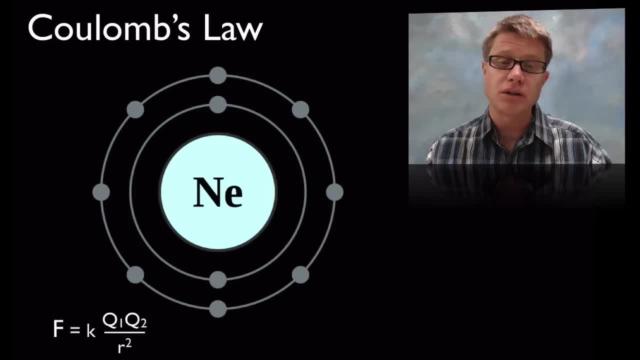 are really going to interact. So Coulomb's law, remember, predicts how atoms are going to interact, And so that's what this example is, Remember- predicted where electrons are going to be. You have these positive charges on the inside and you have these negative charges on the electrons, And 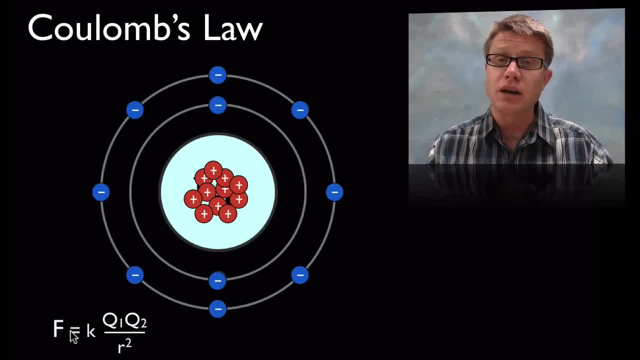 so the larger these charges get, the larger the force holding them together is going to be. But as they move away, as the radius increases, we're going to decrease that force. But there's two problems with that general shell model. Number one: they don't flow in these specific 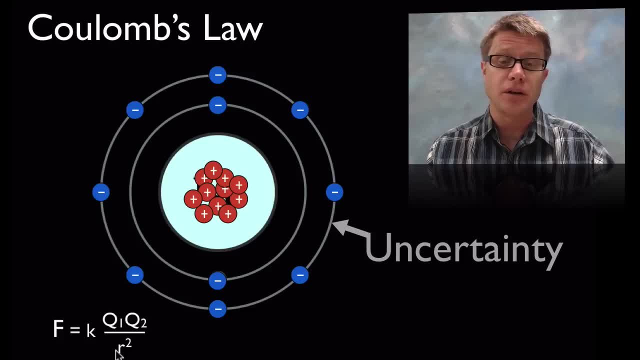 orbits, And that's because of Heisenberg's Uncertainty principle. And then the other one is that spin means we can only have two orbits. So are you really familiar with these two electrons in every orbital? And so this idea of eight in one shell is just not going. 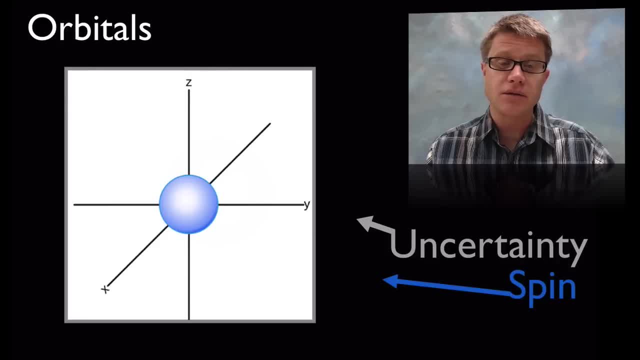 to work. And so there are these orbitals, And if we start on the inside, the first one is going to be called the s orbital, And then we move to these things which are polar, And so we call those the p orbitals. They don't come from polar, but that's how I remember. 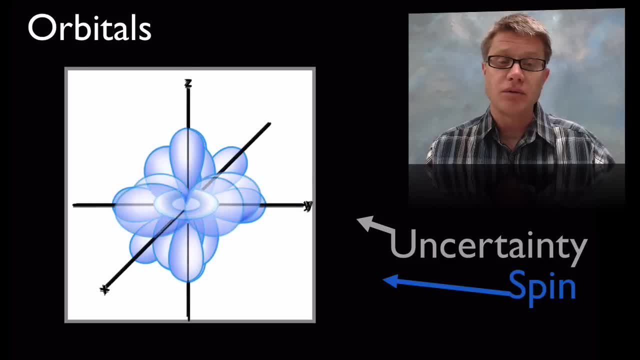 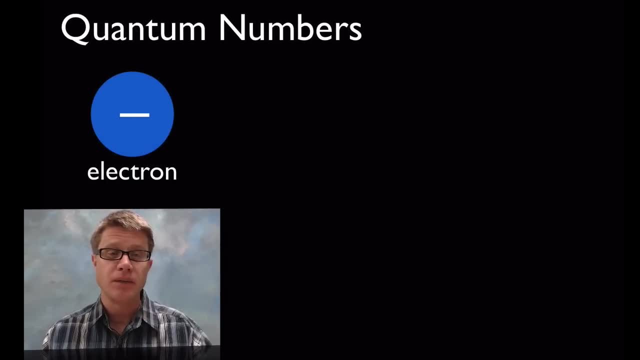 it- And then we move into the d orbitals, And then we move into the f orbitals- I don't know if I have those, But essentially they're all of these clouds of probability where electrons sit, And so we have what are called quantum numbers, And the first three are going to. 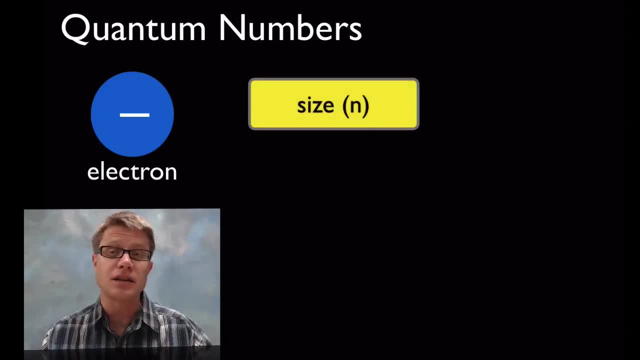 determine what that orbital looks like. So the first one is going to be n, And that's going to be the size of the orbital. As n gets larger, then that area of which those electrons are going to be is going to get larger. We next have l, which is going to be: